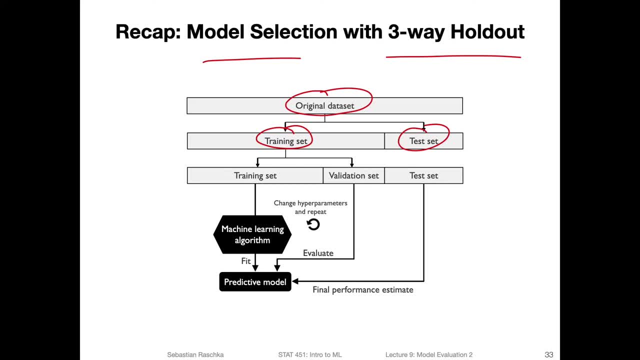 set into a training set and a test set, And then we split the training set further into a smaller training set and the validation set. So we use the training set then together with the machine learning algorithm and a specific hyper parameter set And fit it. so we get a model out of it if we fit the machine learning. 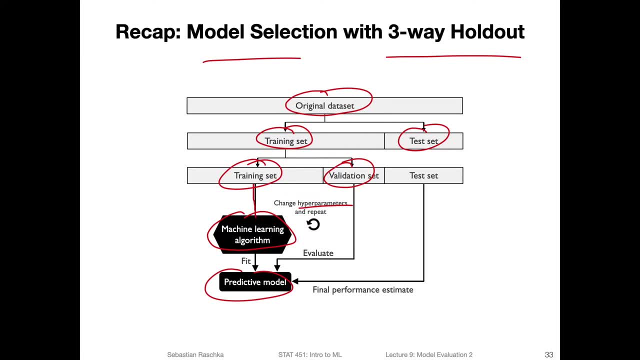 algorithm or the model with a particular hyper parameter setting. And then we do that for different hyper parameter settings and we keep the performances. So we may end up, let's say, with 10 different models, 10 different models and performances, and we select the one with the highest performance. 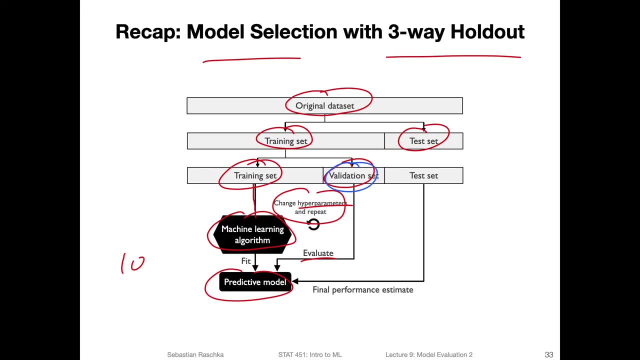 and again, this is measured on the validation set, And when we select the best one, we can then fit it to the sorry, we can then fit it to the combined training set, Or we can just leave it as is and just consider it fit to the smaller training set and evaluate its final. 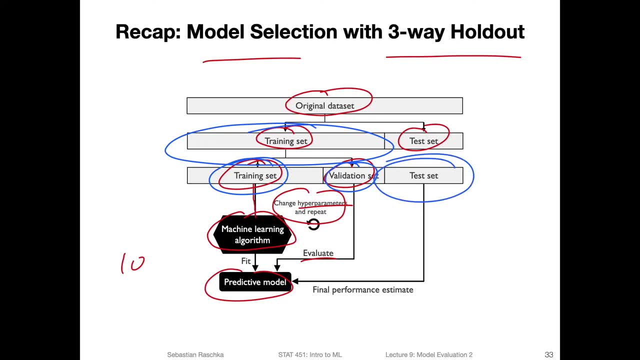 performance on the test set. So why do we have an independent test set here? It's because when we do this procedure here, we change the hyper parameters and we evaluate many different models. So there can be some sort of selection bias if we select the best performing model. 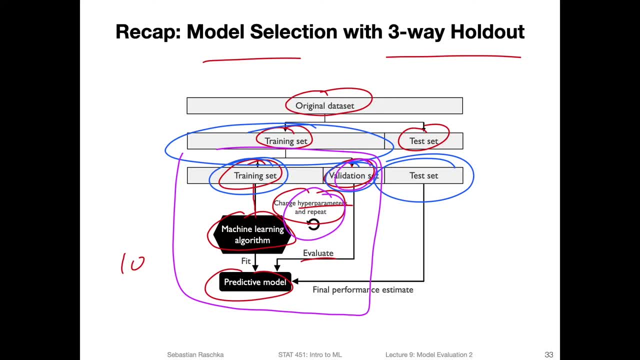 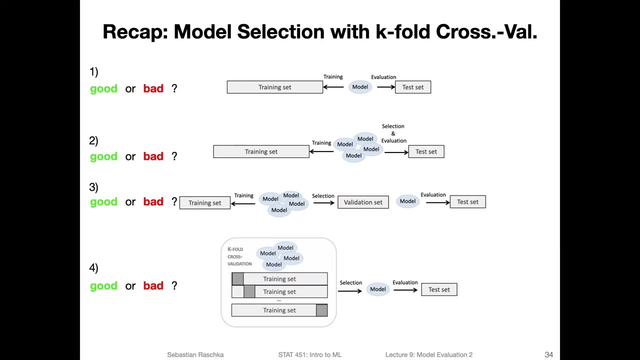 Okay, so here's another recap. I made this figure some time ago. I never really used it anywhere, So I'm just recycling this figure here on my phone or my computer. So it's just, I think, a useful way to recap the model selection case. So I'm just going to. 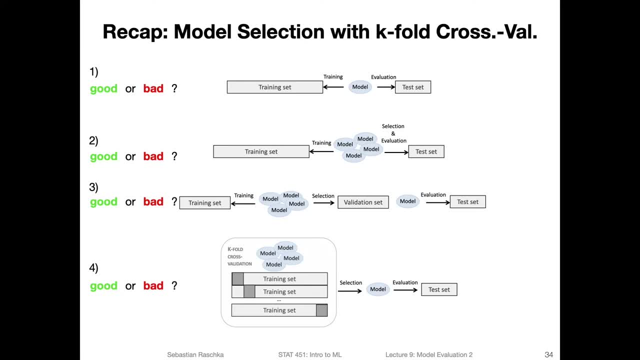 recycle this figure here on my phone or my computer. So it's just, I think, a useful way to recap the model selection case. So let's see what we have here First. what we have here is the scenario where we just evaluate a model. So so we have a model that is fit to the training set. 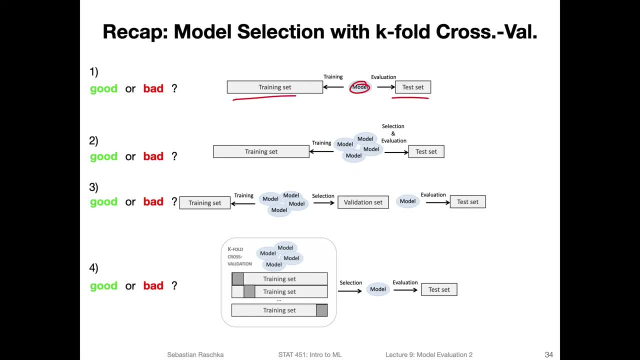 and then evaluated on the test set. but we have no model tuning. So in this case, if we don't do any model tuning, just using a single training set in a test set is absolutely fine. So that's a good approach. There's nothing wrong with this For the 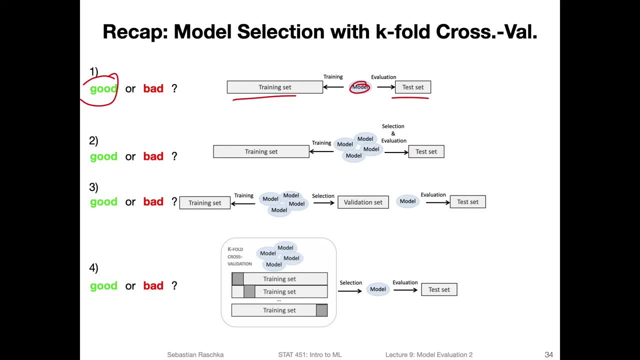 second case, what we have here, that would be a case where we have multiple models. we have a training set and a test set And we train all the models here, let's say, with different hyper parameter settings on the same training set. And then we 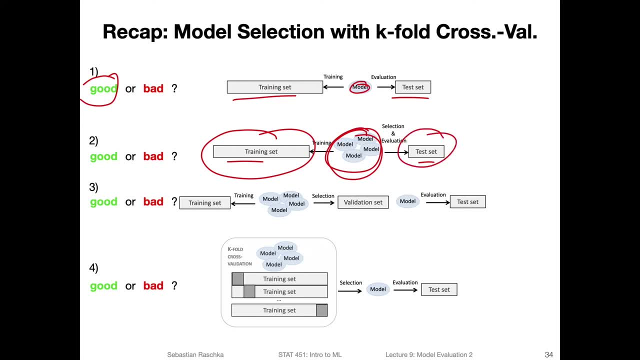 evaluate all the models on the same test set and we use the best performing one. This is actually not a good approach because, yeah, we shouldn't use the test set multiple times. the test set should only be used once. In step three, this would 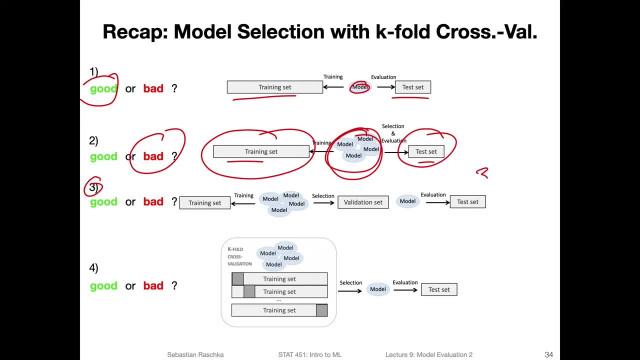 be. if I look at it, this would be the three way method- Holdout method that we talked about just one slide ago. So we have again multiple models fit to the training set. they have all different hyper parameter settings, So the algorithm was run with multiple hyper parameter settings. So we 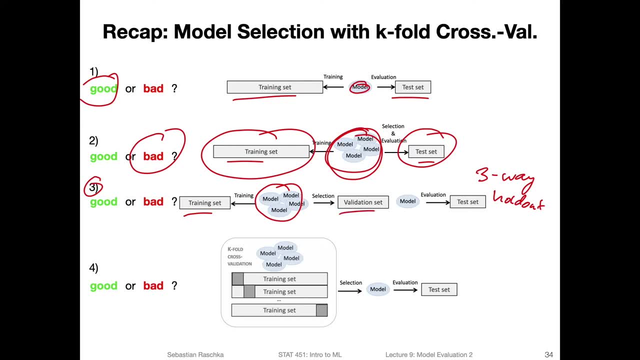 get different models And we use the validation set to select the best performing model, which we then evaluate on the test set. So this is also a good approach. That's what we talked about last time. So we avoid the selection bias, or we 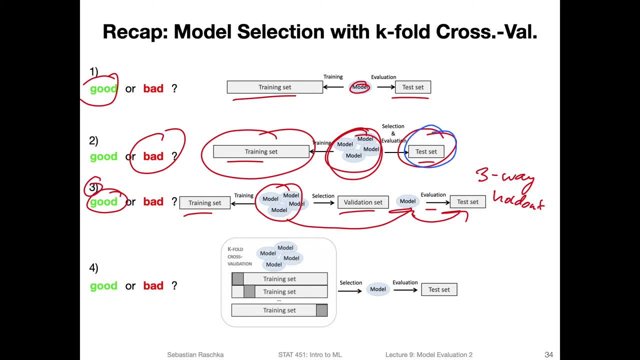 avoid biasing the performance estimate on the test set by using this validation set to rank the models. A better way would be K Ford cross validation, which we talked about last week. So this would be even better than the step three, three way holdout. 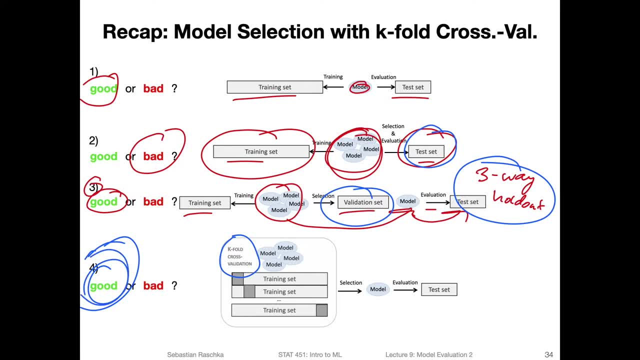 method. So I would say go with method four instead of three, especially if you don't have a very large data set For deep learning, it may. it's totally fine to use three, because we usually have larger data sets And in deep learning there's also 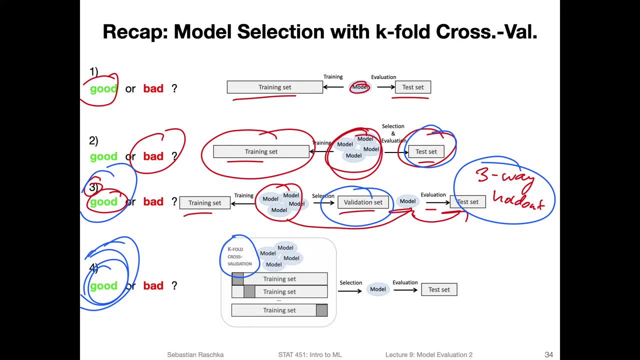 the added complication that we have to kind of sometimes babysit the models and see whether they converge when we fit them. Okay so, but again to recap, K Ford cross validation. So we now, instead of creating our validation set, we have the different rounds and K for cross validation when each round we 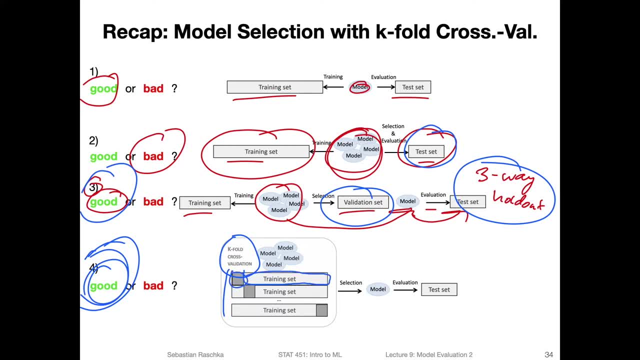 fit the model to the training set and then evaluate it on the validation set. And we do that with different hyper parameter settings. So if we have four hyper parameter settings, we get four performance estimates from that And then we select the best performing hyper parameter setting based on the K Ford cross. 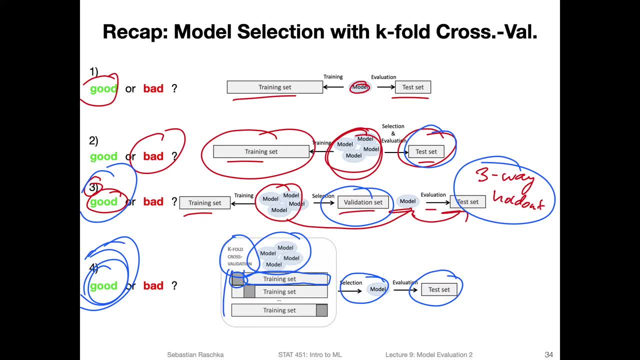 validation performance and then evaluate that model after fitting it on the combined on the whole training set. Then we evaluated on the test set. So this was the K Ford cross validation that we talked about last week. Now we will go a step further, So 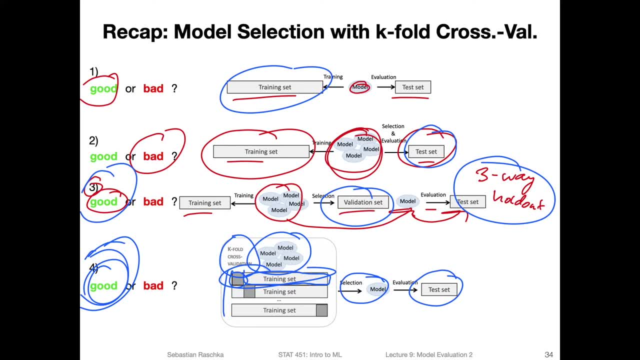 talking about this. this really for selecting hyper parameters. So now the next task would be selecting algorithms. you can think of it as another loop, So you can think of this as hyper parameter tuning, for oops, can't really write down here, because there's my color- 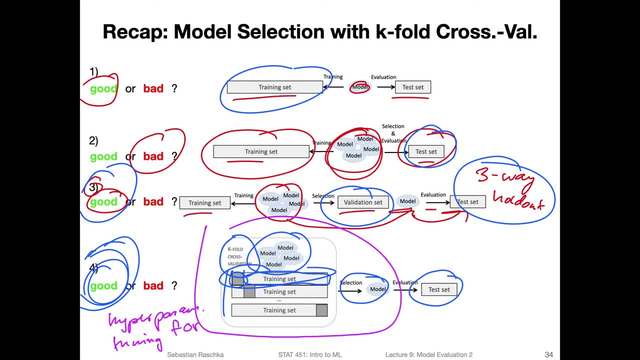 bar for the pen hyper parameter tuning for given algorithm. So that's what we do here. Now we want to take a further step And we want to compare different algorithms. So this could be, for example, for K and N. But now let's say we want. 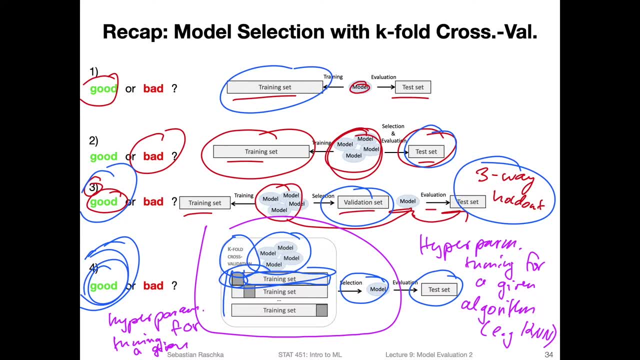 to compare K and N To decision trees, to gradient boosting, to random forests and so forth. So we want to compare different algorithms And each algorithm will also include this hyper parameter tuning, because we really want to select the best model from each algorithm and then compare them to each other. So what we do is we add: 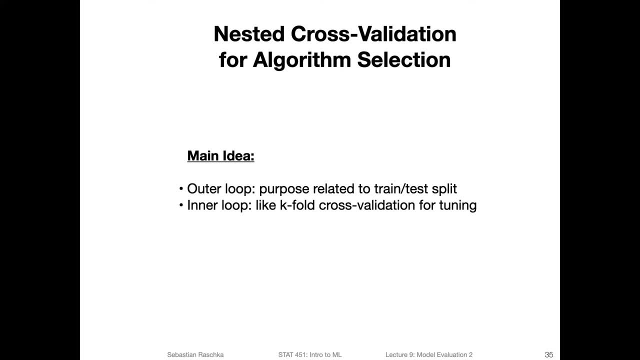 another loop to the cross validation procedure, which is why it's called nested cross validation. So we have an outer loop And the purpose here the same purpose as doing the train and test split. So the outer loop is really like for getting the performance of a. 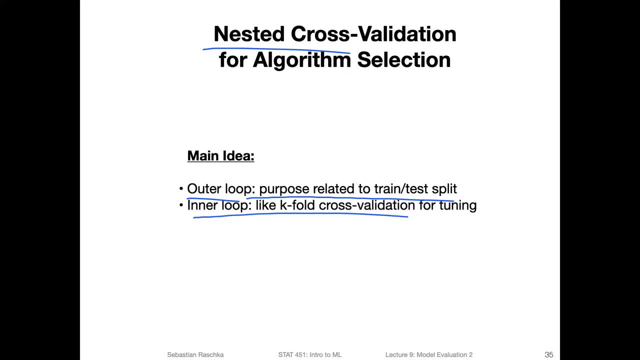 model, whereas the inner loop is more like for the hyper parameter tuning. So we have an inner loop that is like K for cross validation for tuning. So here it's not for finding the best model or hyper parameter setting, And and then the outer one is for evaluating. 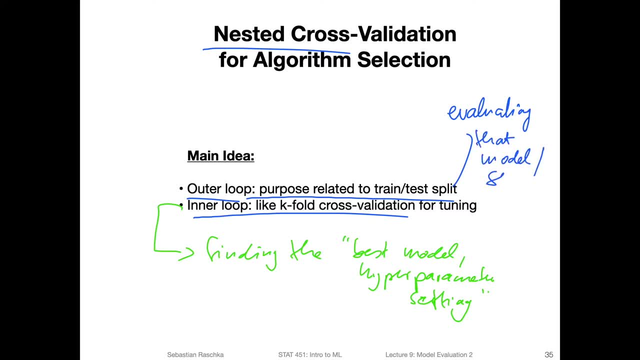 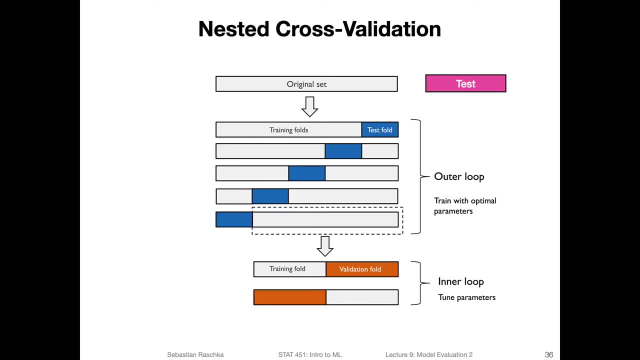 that model or say, hyper product setting. So there are now two. it's a two step procedure in a sense. in essence, Yeah, because it is a two step procedure. it's a little bit bit more complicated than our regular k fold cross. 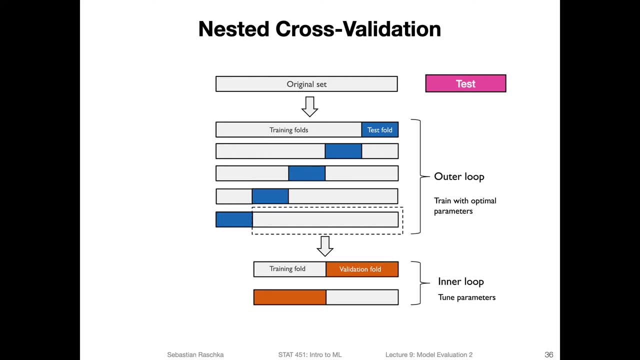 validation. In fact, you can think of it as two k fold cross validations nested within each other. Okay, let's try to go through this illustration in a way that is the least confusing, starting at the top with our original data set. So we have. 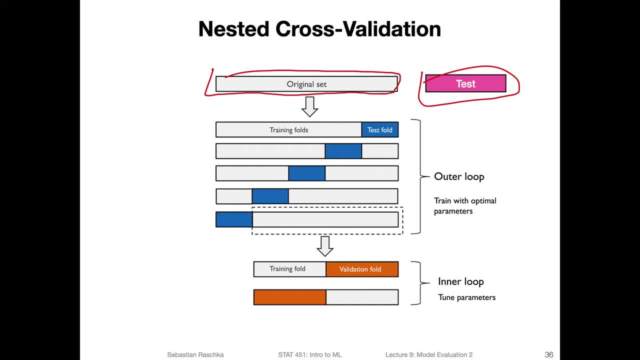 our original data set. assume we also for later have another independent set for testing, but this is our main training set. So what we do is we have similar to k fold cross validation, the loop that we have like a five fold loop, like in favor of high fold cross validation, And in each round 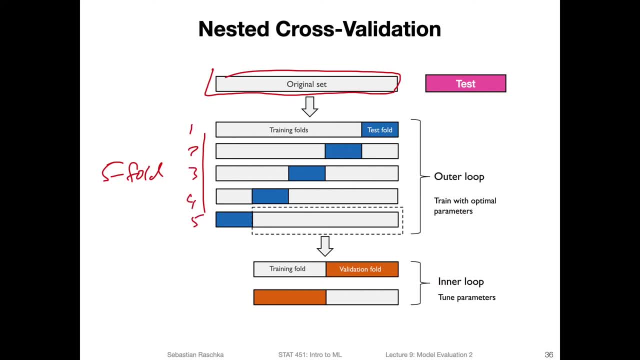 here around 12345, we split the data set into training faults and a test fault. So this is the- for this case the computer combined training faults for the first iteration and then the test fault. So we do that five times. But now, in contrast to k, 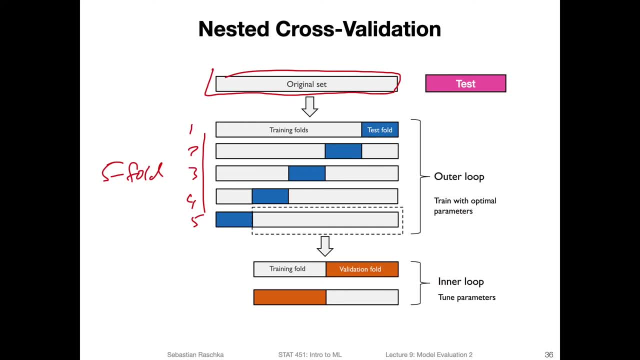 fold cross validation. So in k fold cross validation, what we would do is we would fit the model on the training faults and evaluated on the test faults. Here we don't do that. we go one step further. So we take a training fault. So here let's. 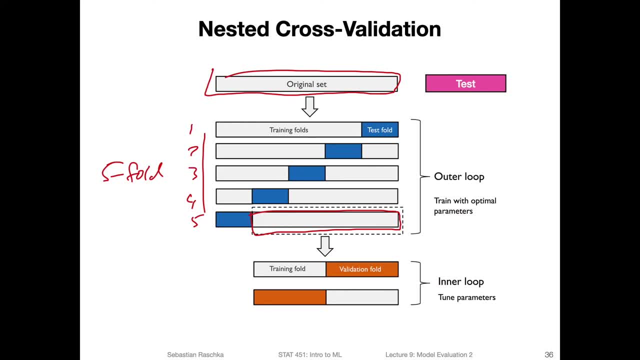 consider this case here at the bottom. it's easier because I attached something to the bottom, This one. So this is again our training fault, And here what we now do is we do another k fold cross validation. So instead of 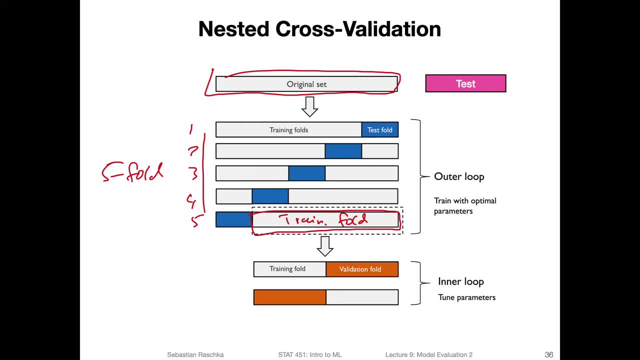 fitting the model on this one and operating on the test fault. we have no two fold k fold cross validation. So in this case many people do a two times two cv nested cross validation. sorry, two, five times two nested cross validation. But 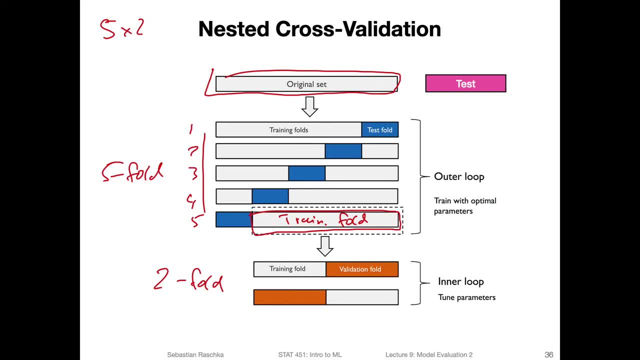 yeah, I experimented with that. Um, there's no reason really to do the five by two. it can also be five by five or five by 10.. So, based on my experiments and experiments by a student of mine, Richard Yang, we didn't. 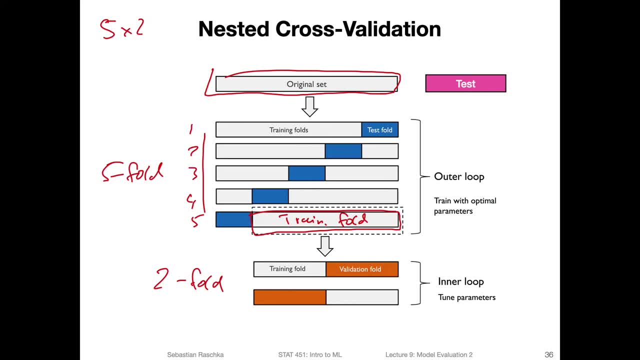 find any substantial advantage of having more accurate estimates when doing a five times two procedure, versus five by five or five by 10, or two times five and so forth. So in different data sets it's different. So it was not like as. 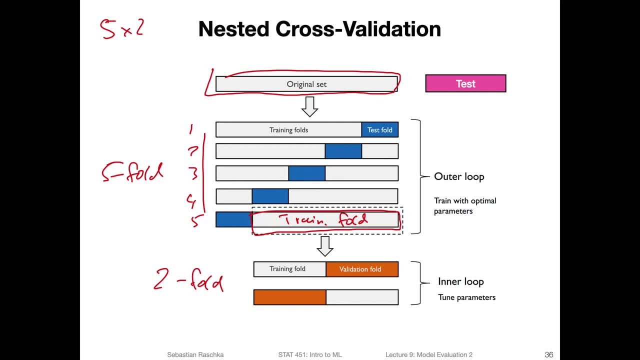 clear, as in Ron co Harvey's paper, where 10, fold cross validation on most data sets was better than five fold or 20 fold. we didn't find a trend like that, But in any case. so let's consider the five by two procedure. So now we have. 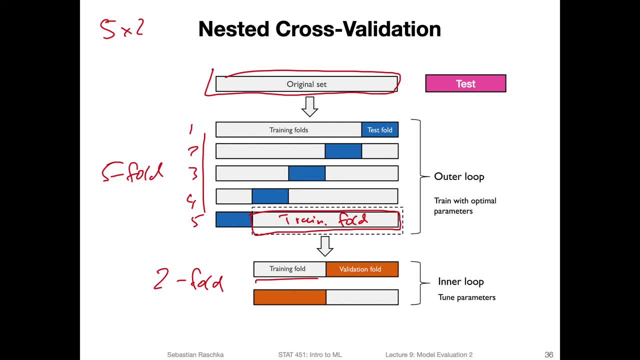 split the training fold further, So we have a smaller training fold and the validation fold here. So here this is really like the inner loop is really the one that is most similar to k fold cross validation for model selection. So here I also. 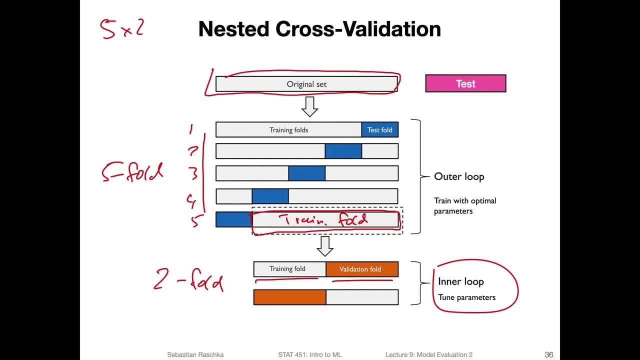 should say: let's say we talk about decision trees, we apply a decision tree algorithm to this whole nested cross validation procedure And then in the inner loop, in the two fold procedure, we do the hyper parameter tuning. So we would evaluate, for example, the 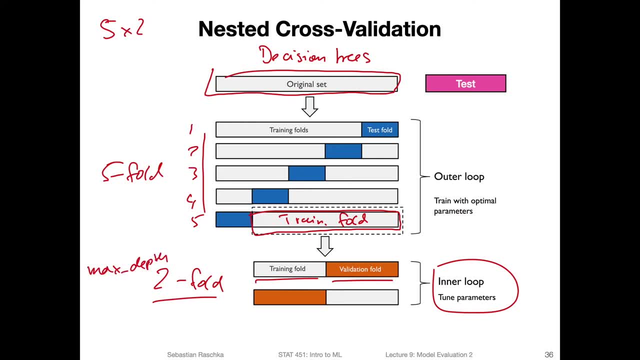 max depth of the decision tree on the criterion like entropy or Guinea And so forth. So in each one here we would tune the hyper parameters So we would for example find, based on this inner fold, that a max depth of two and entropy would be best. 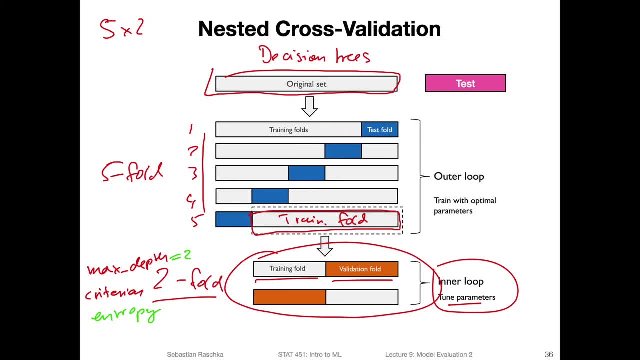 So we know that then and then we would fit the model with the setting. So we would evaluate many different hyper parameter settings back in K for cross validation And then for the best one we would fit the model on the training for them with a. 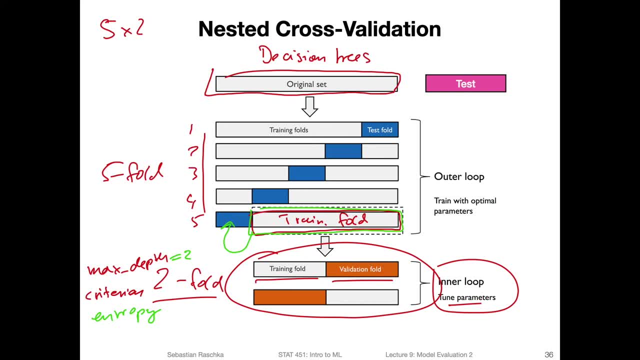 best settings and then evaluate it on the test fault. So now we have done that, for for this last round here, we found that to max depth of two and entropy is best And we have the performance of that for the test. for, let's say, it's 80% on the test fault. Okay. 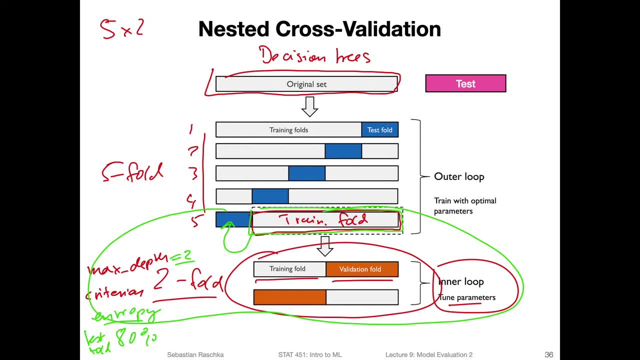 next, then we would do that again. Now let's say, let's say, let's say, we do that on on this case. here we can just take this one. it's just a little bit harder to imagine it because we 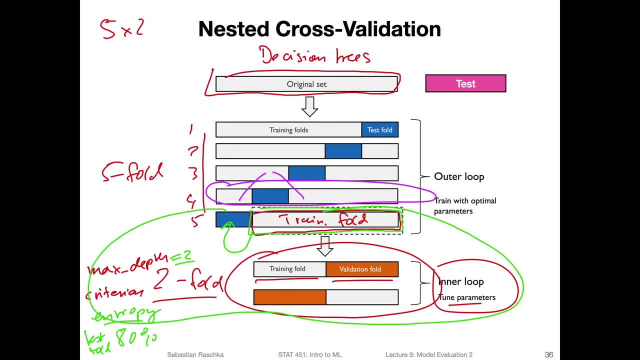 have the training faults here on both sides. So when we combine them this would be our training set. So here we would again split that into smaller training fault and validation fault and then do hyper parameter tuning And based on the hyper parameter 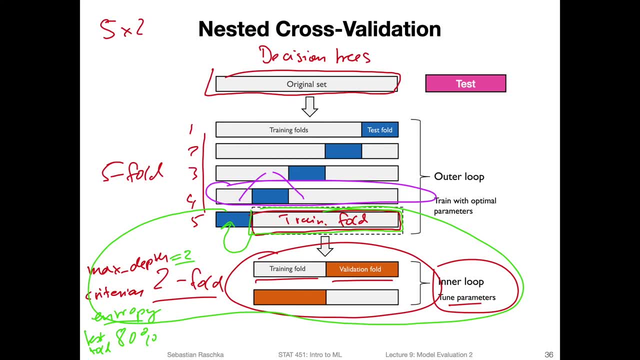 tuning, we also would find the best settings. It can be. that's also, that it's also the same, that it's consistent. that's max depth of two and entropy, But in practice it may be something different. it could also be, let's say, max depth of. 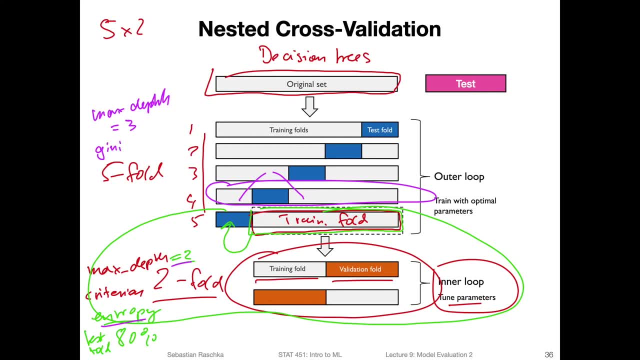 three and no, it could be Guinea, And then we would get the performance of that one on this test fault. So we do that then five times. we hope if we have a stable model, then all of these suggest the same best hyper parameter settings and we 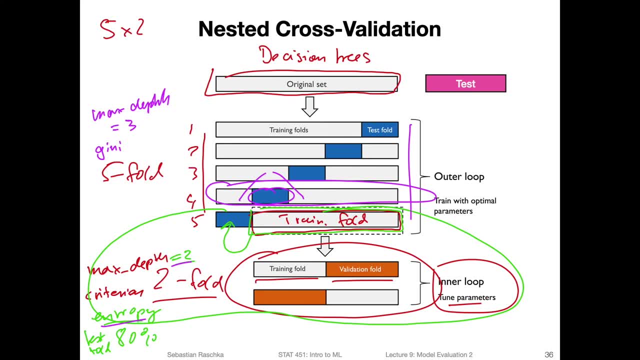 evaluate them on a test fault, But that does not have to be true, And that's why it's more like an algorithm selection procedure, the nested cross validation. So here we finish this then. So we do this for the five iterations And we 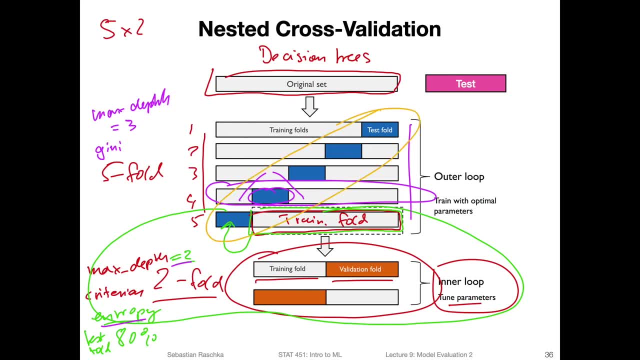 will get five performance estimates. So five performance estimates, And they can be from different models, So we would then average those. So we would, in this case, let's call them: i equals one to t for t test fault, And then we would average, for example, the: 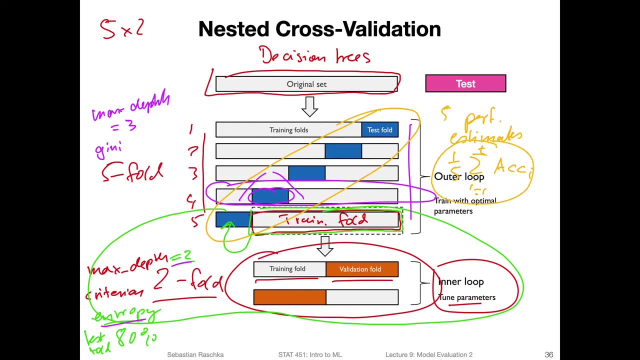 accuracies, And we do this then for the decision tree. So we have a accuracy of the decision tree algorithm on that data set of, let's say, that's averaged 83% or something like that. So we have evaluated now the decision tree algorithm on that. 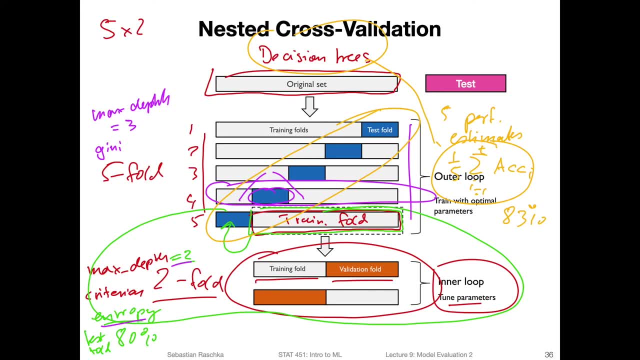 data set. Now then, after doing that, we can do the same thing for different algorithms. we can, for example, use KNN or gradient boosting or random forests, and repeat the procedure, And for each of them we get an accuracy- let's say 84.. 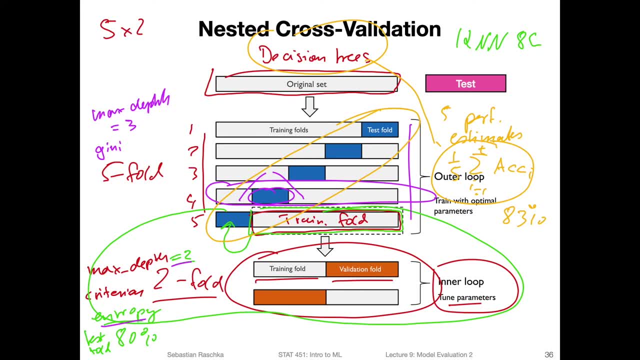 Let's do something that's maybe more substantially different. say 80%. So it tells us that if we would use an algorithm like KNN and we tune it to a given data set and things like that, we would expect that it gets roughly that performance. So after we selected: 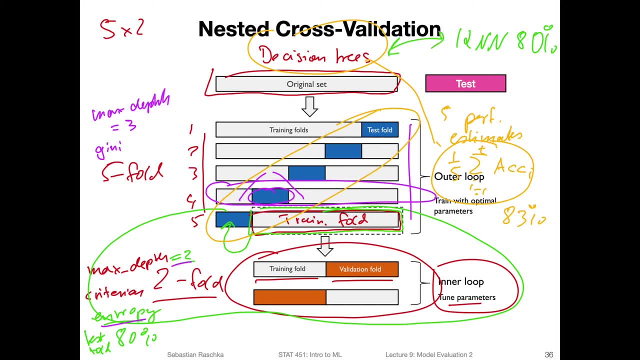 our algorithms. so if we compare, let's say, decision tree and KNN to each other, so based on these just been comparing which one has the higher accuracy- we can then pick this algorithm. let's say we end up picking the decision tree. 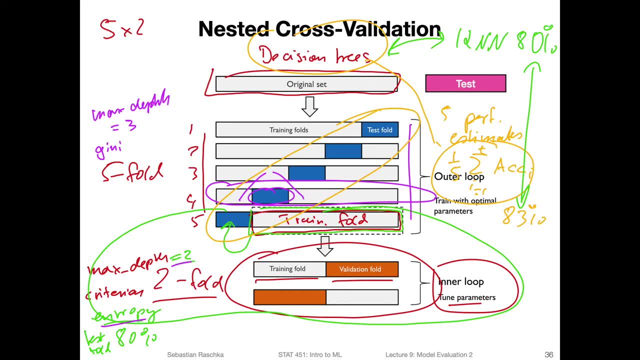 algorithm as the best algorithm for this data set, then we still don't have a model. if we need a model for application, If we wanted to get a model, we can take a look And the different hyper parameter settings across these five folds, select the one that more that had either the highest. 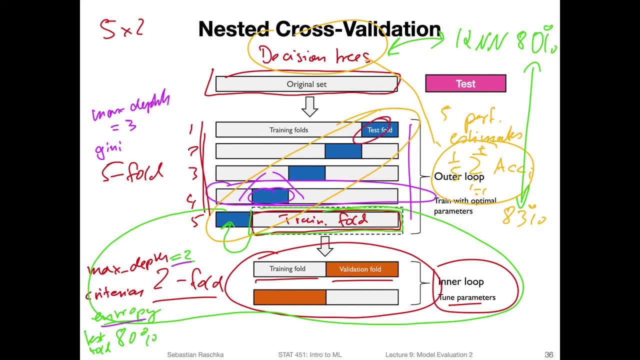 test performance here on the test fold or, if we have ties, select the one setting that was most often selected and then fit a model on the whole data set with the setting and evaluated on the test set to get a independent performance estimate on the independent tested estimate of the. 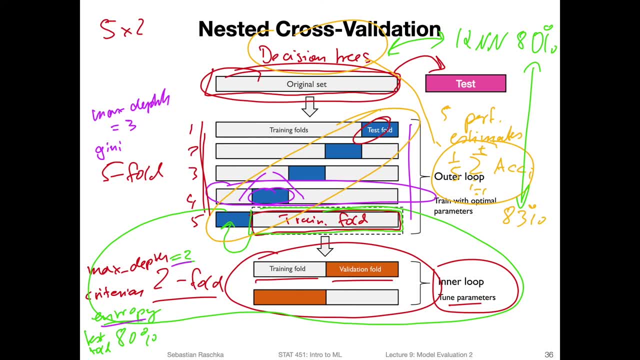 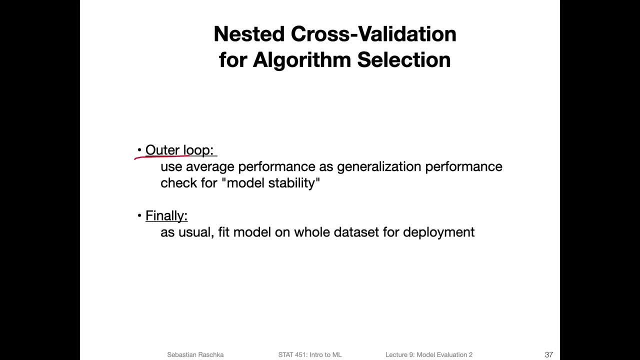 generalization performance. But yeah, in a nutshell, this is how the nested cross validation procedure works Yet. so just a recap, the outer loop here. So we use the average performance as generalization performance. it should be one point. Another point is that we can also use that outer loop to 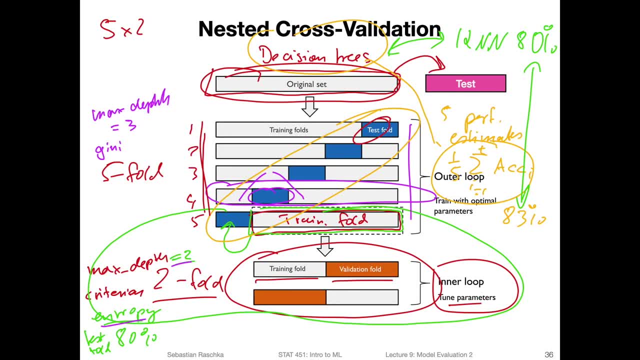 check for model stability. By that I mean we can look at what the variances of these estimates and also we can see how different the different settings are. So if there's a large variance, it also is something that may concern us. So if we consider the case, 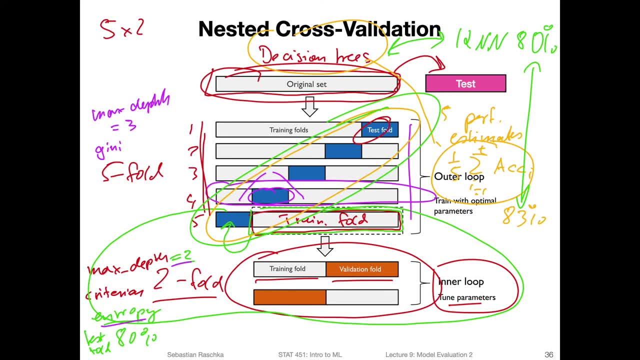 where we have the archive sanity per server server. we don't want to choose an algorithm here that is very unstable. that has sometimes a good performance, on some cases here really bad performance, because then it's really like some users have a really great experience, Some users have a very poor. 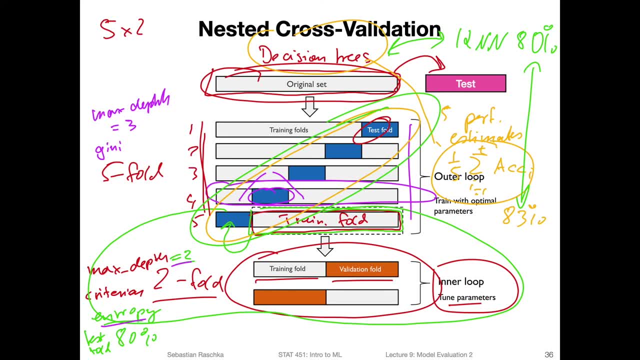 experience. So it would be better, even though maybe on average the performance is lower, to pick an algorithm where the settings here vary a little bit less and where the performance estimates are a bit more stable. Okay so, and then, after we've done that, we can then fit the model on the. 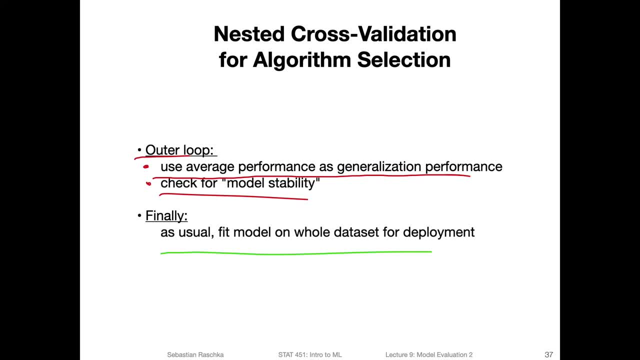 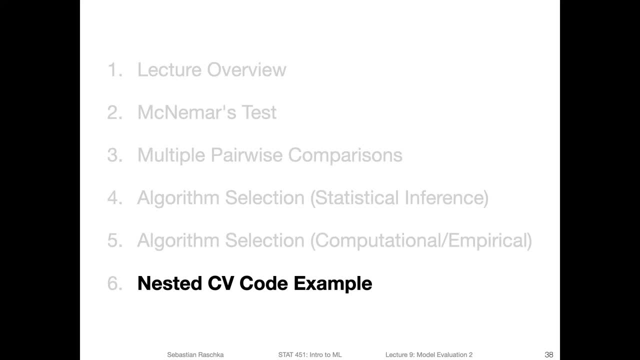 whole data set and get it ready for deployment. Alright, so the next video, then the last video for this lecture. like promised, this will be a little bit of a shorter lecture week because of Thanksgiving. In the next video I will also show you how we can.